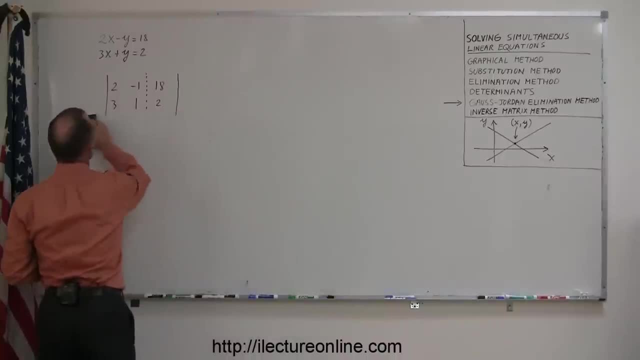 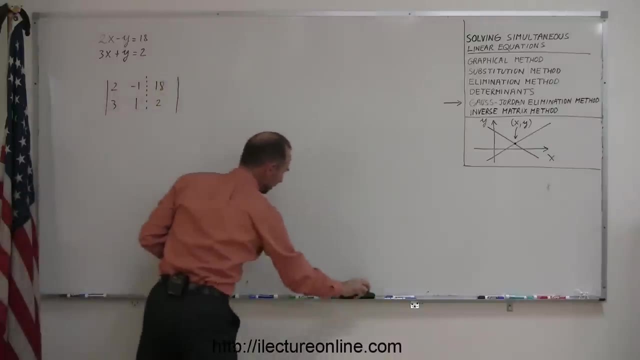 And I probably got a little bit of time for that- Got a little bit carried away, Made it a lot bigger than it needed to be, so let me make it a little bit smaller. So there we go Now. the whole idea is you're going to go through a set of steps, a set of operations. 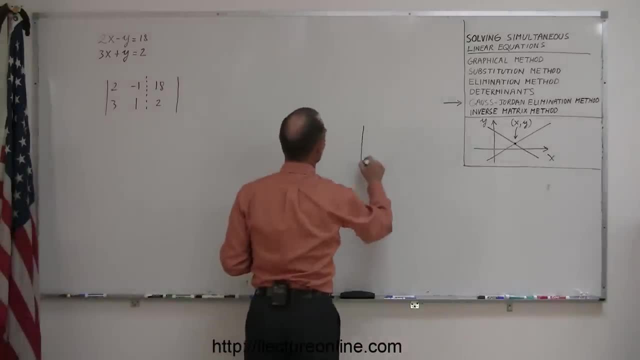 in such a way that at the very end, when you're all done, you end up with something that looks like 1, 0, 0, 1.. Oop, nope, not like that. It looks like this: 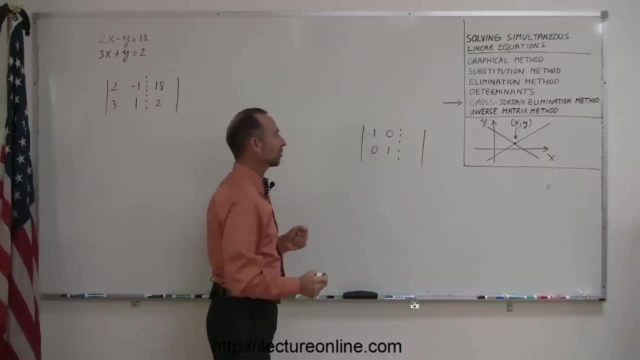 so you end up with a one across the diagonal, zero in the other direction, and then the value for x and y will be over. here you can actually, when you get to this stage, read the actual solutions, the two numbers representing the x and the y coordinate of the points where the two lines cross. 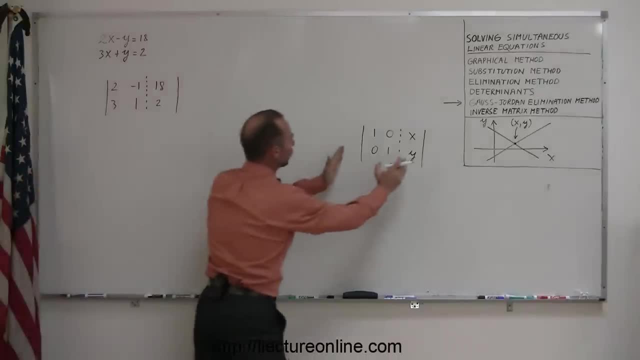 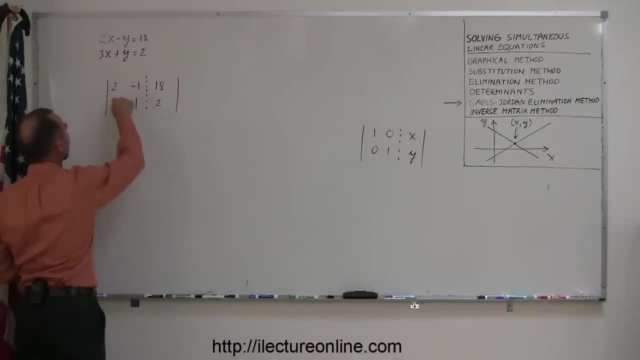 so the question is: how do you go from here to here? well, you go, do it in a very systematic way. you go to each number first and change it to the form that you want. you start with the upper left corner, right here, and you want to make this number look like this. in other words, you want to make the 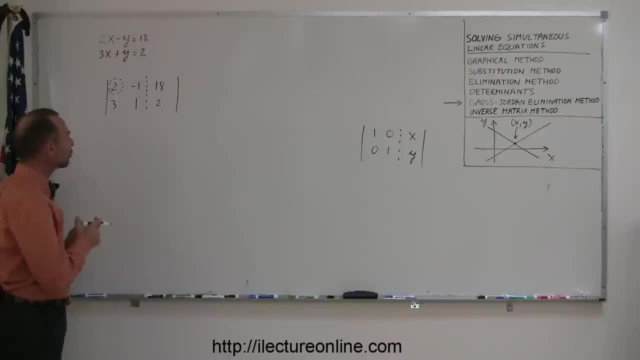 two into a one and whatever you do, you have to do the same thing to the entire row, to all three numbers in that row. so to make a two into a one have to take the very first row and divide it by two, because then the two will divide into two. 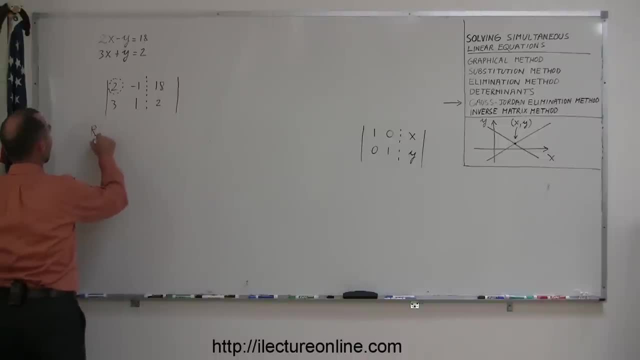 then turn into a 1.. So I'm going to take the first row, row 1, and change it to half of row 1 or replace it by half of the original row. In other words, I'm going to take every number and simply 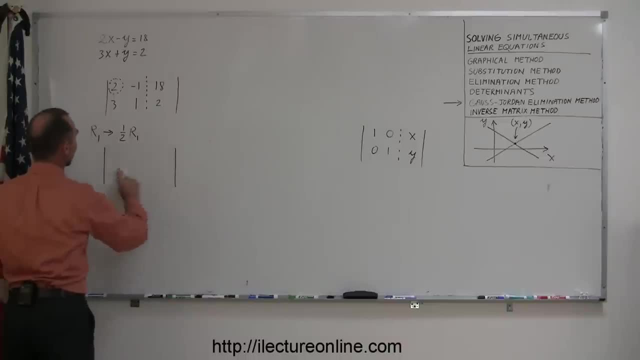 dividing it by 2.. When I do that, I get the following thing: I don't do anything to the second row, so that stays as a 3, a 1, and a 2, but I take the 2 divided by 2, I get 1.. I take: 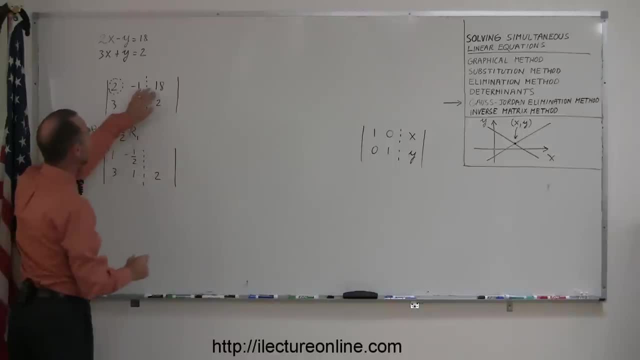 the negative 1 divided by 2,, I get a negative 1 half. I take the 18 divided by 2, and I get a 9.. So I'm partway there. I turn the 2 into a 1, and I have what I need in that particular location. 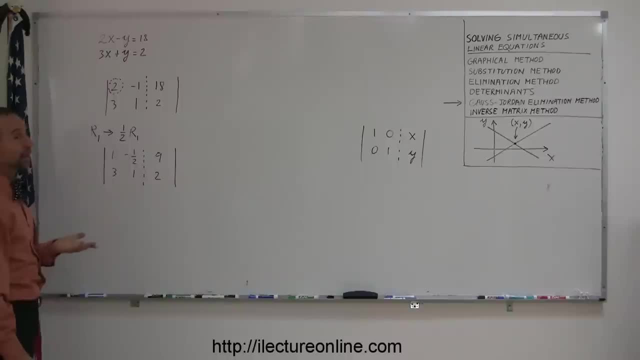 The next thing I want to do is turn the 3 into a 0.. How do I do that? Well, the technique is: you take the second row and replace it by the negative of this number multiplied times the first row. So I take the negative of this number. 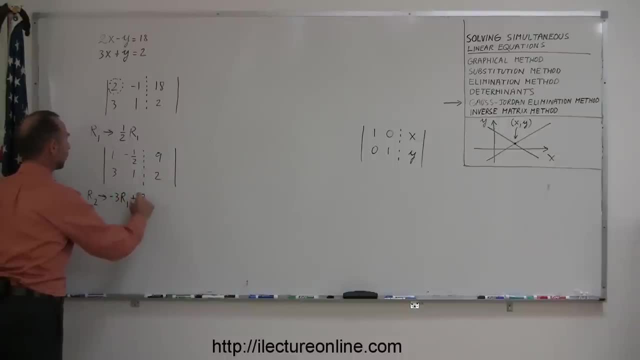 negative of this number and I take the 2 divided by 2.. So I take the 2 divided by 2, and I get a 3 times the first row and add it to the second row, and I do that for each one of. 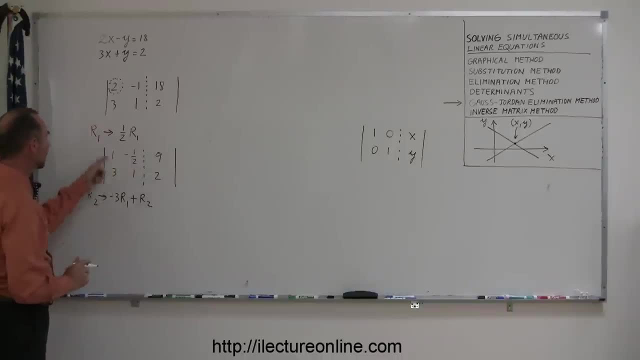 the three numbers. so negative 3 times a 1 is negative. 3 added to 3, I get 0. so nothing happens to the first row, so I can rewrite this one as is. so I take negative 3 times a 1. that's negative. 3 added to 3, I get 0. negative 3 times the. 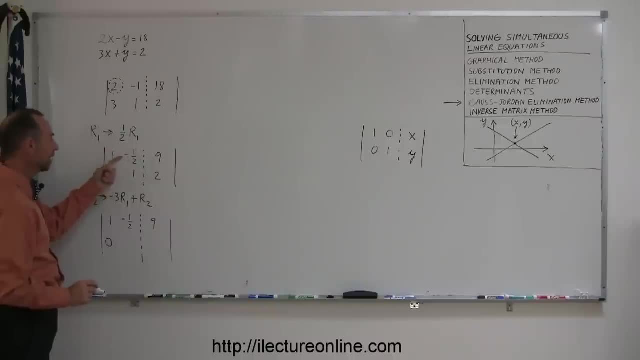 negative. 1 half, that's a positive 3 halves. added to 1, which is 2 halves, that gives me 5 halves, a negative 3 times a. 9 is negative. 27 added to 2 gives me a negative 25. I'm halfway there now, because now I turned this number into a. 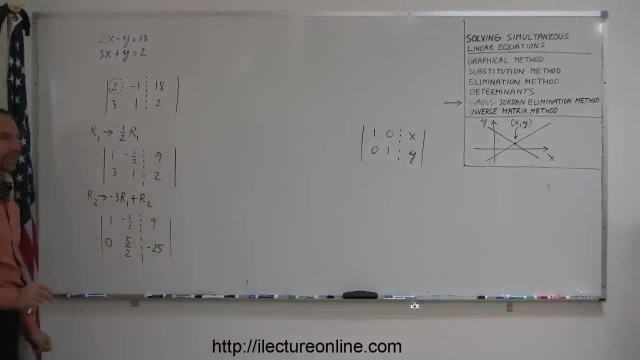 0. so I have the very first column as a 1 and a 0. in case you didn't quite get how that worked, let's do it again. I want to take a 3 and turn it into a 0. the technique we use is we take the negative. 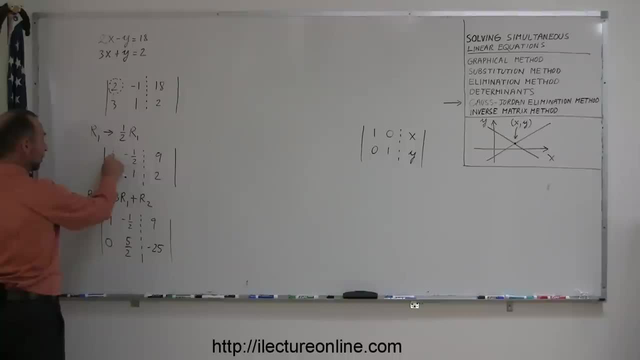 of this number. multiply times the first row, where the 1 is so negative. 3 times 1 is negative. 3 added to this number and we get a 0. but since I did it to the first one, I need to do it the second and the third number as well. so I take: 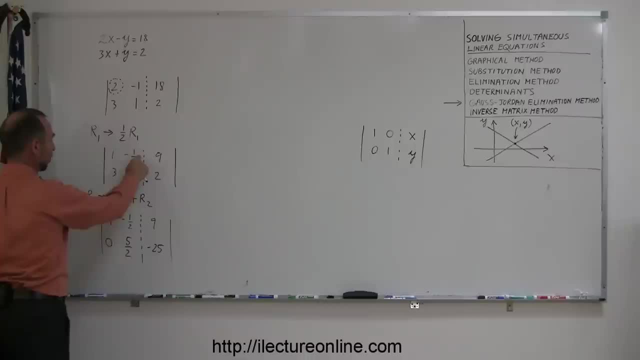 negative 3 times the number in the first row. negative 3 times a half is a positive 3 halves plus 1 is a positive 5 halves and I put it there. for the third number, it's negative 3 times a 9, which is a negative 27 added. 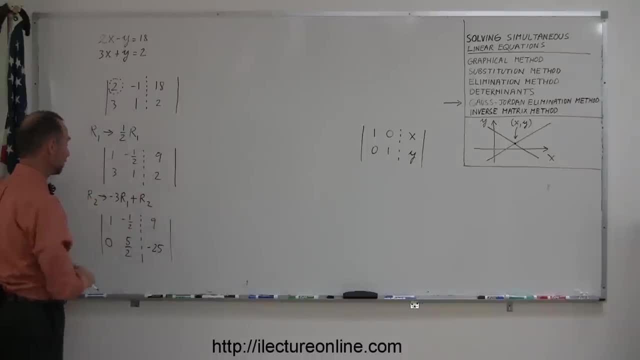 to 2. negative 27 plus 2 is a negative 25, and I'm done, all right. the next step is: I want to get this number to be a 1, so I move over to the second column. I go to where I need a 1, and that's in this location. right here, I want to turn this. 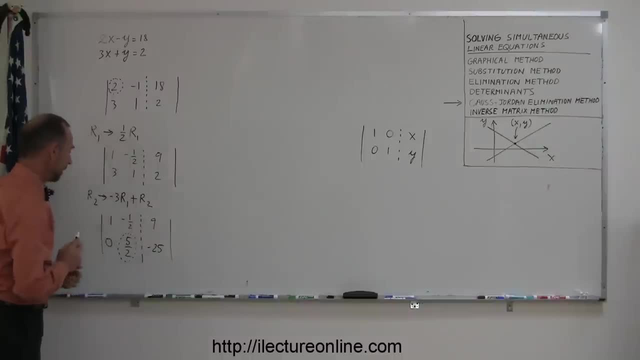 number into a 1. I can do that by multiplying this by its reciprocal. if I multiply this by 2 fifths, this will turn into a 1. of course I multiply this by 2 fifths, have to multiply this by 2 fifths, so the 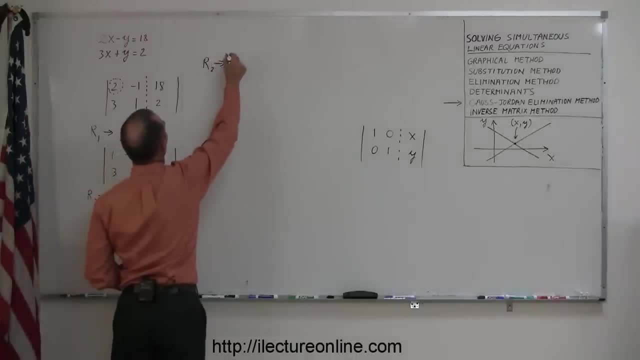 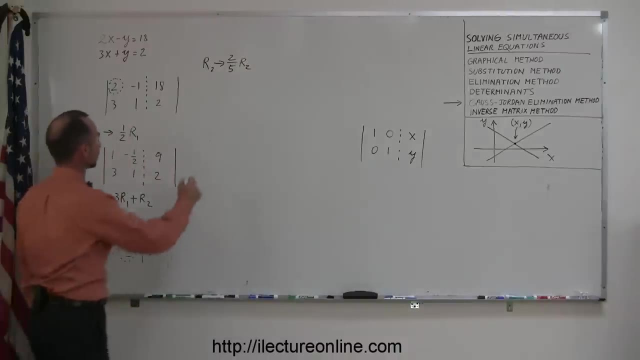 technique is: take the second row and replace it by 2 fifths the second row. in other words, I'm multiplying the second row by 2 fifths. if I do that, I get the following notice: since I'm only changing the second row, nothing changes in the 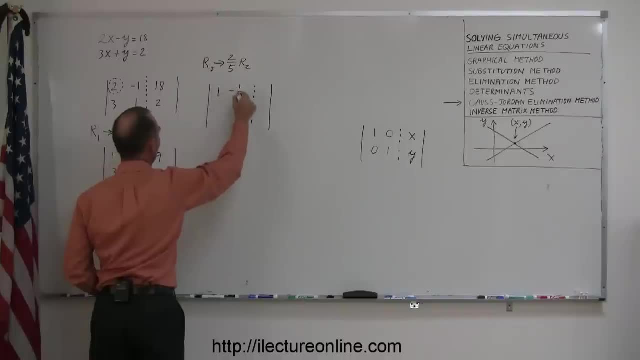 first row. so this stays as a 1. a negative 1, half a positive 9. but here in the second row, of course the 0 doesn't change, because I can do anything to 0. it stays as a 0. multiplying this by 2, 5th, that becomes a. 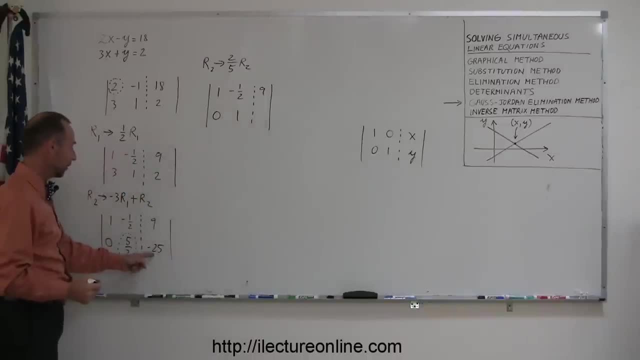 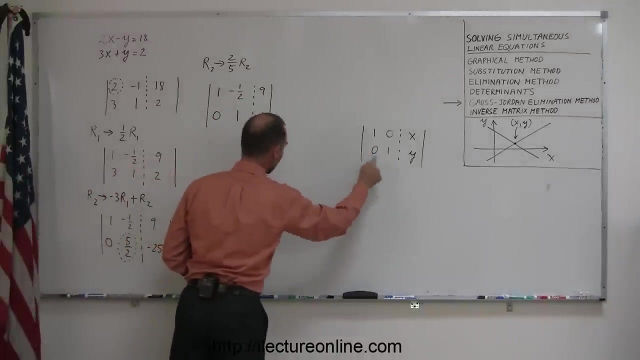 1 and multiplying this by 2, 5th. well, 25 divided by 5 is 5 times 2 is 10, and since it's negative, this becomes a negative 10. I'm almost there. notice that these three numbers now look like these three numbers over here. the only thing left is: 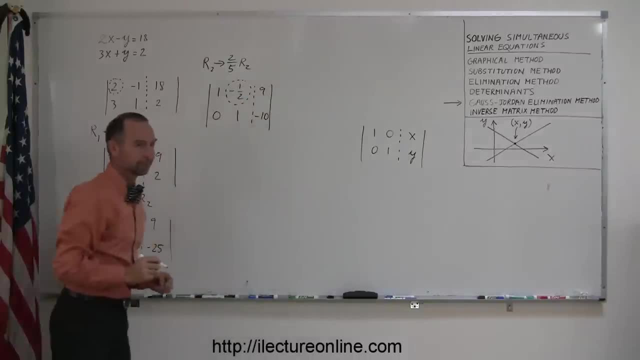 I have to take this and turn it into a 0. so to do that, I take the first row and replace it by the negative of this number, which is a positive 1, half times the row that has the 1 in it, which is row 2, and I add it to the row that I'm 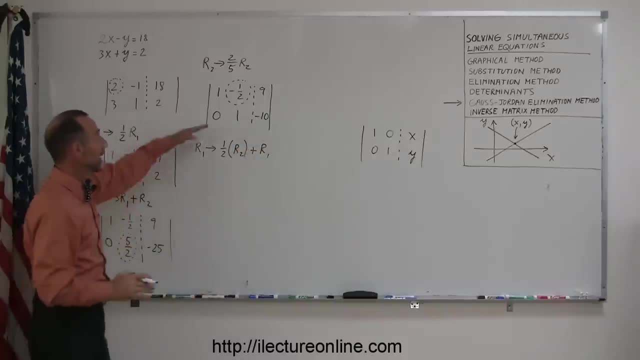 changing row 1. of course I have to do that to every number in the first row. so what happens? I'm not changing the second row at all, so that stays as 0, 1 and minus 10. if I do this to the first one notice, nothing changes. if I take 1 half times row 2, that's 1. 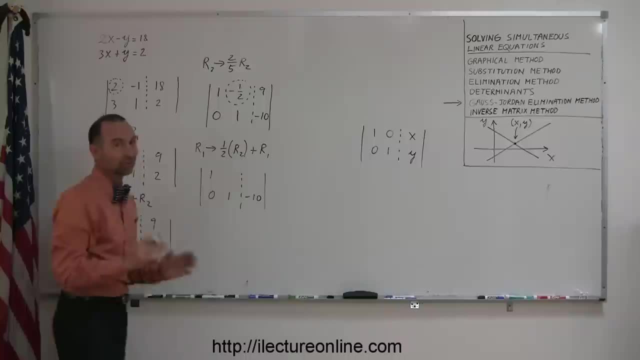 half times 0 and add it to the first one, the 1 doesn't change, and that's the technique. is designed to do that, not to change what already accomplished. but notice for this number right here, if I take 1 half times the second row, which